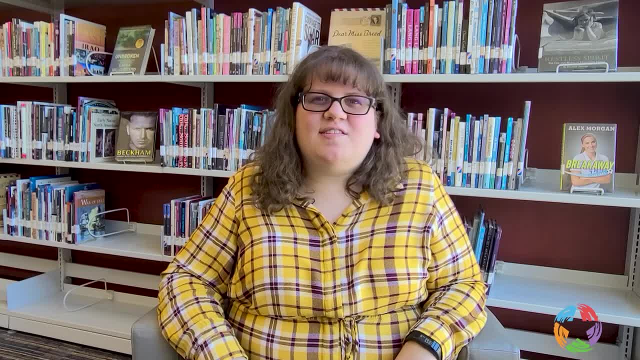 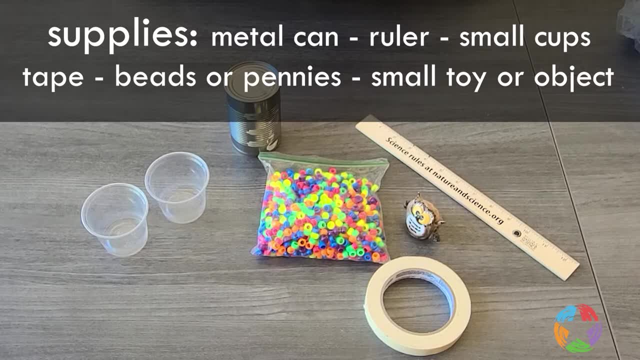 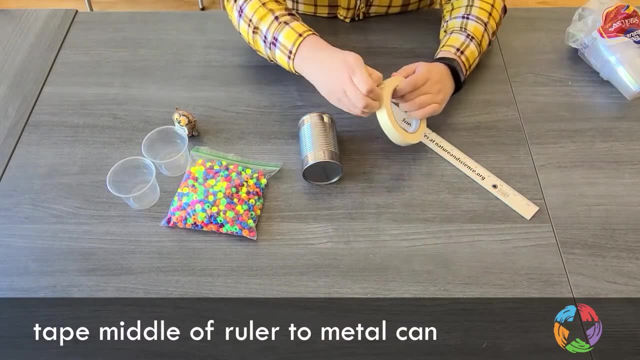 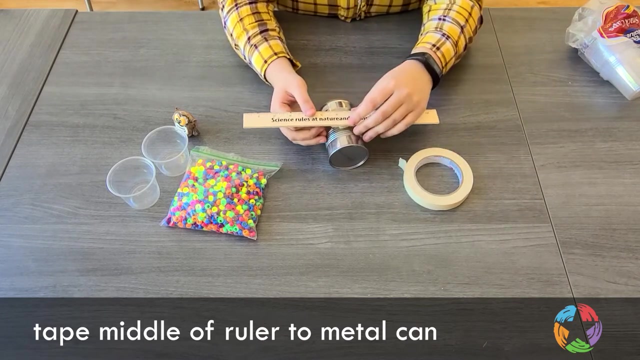 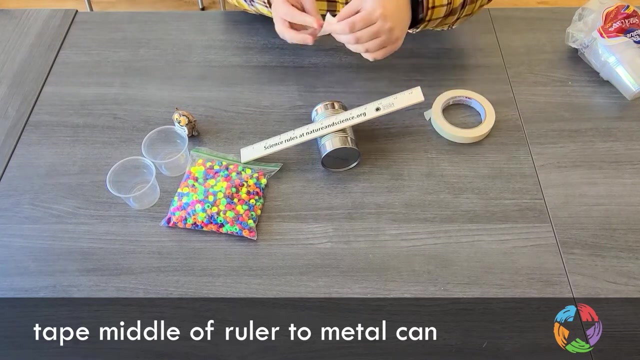 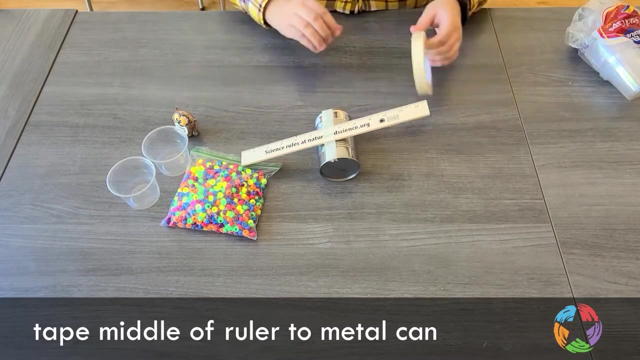 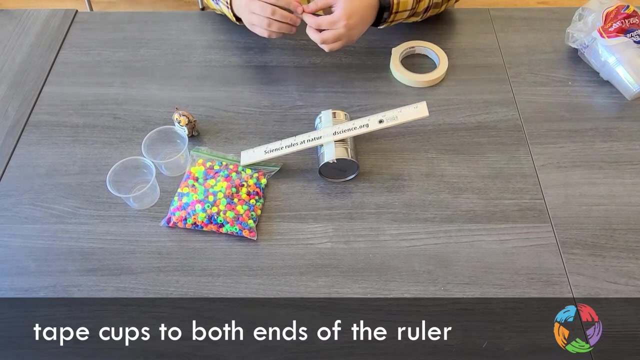 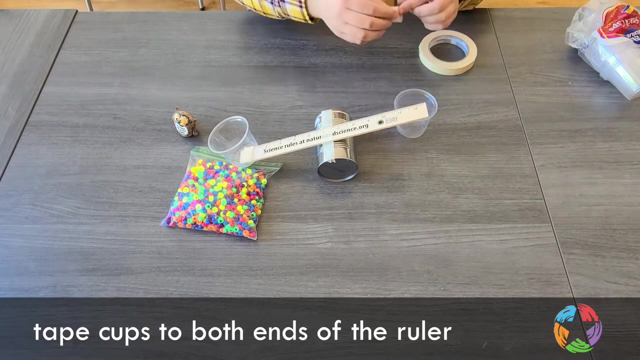 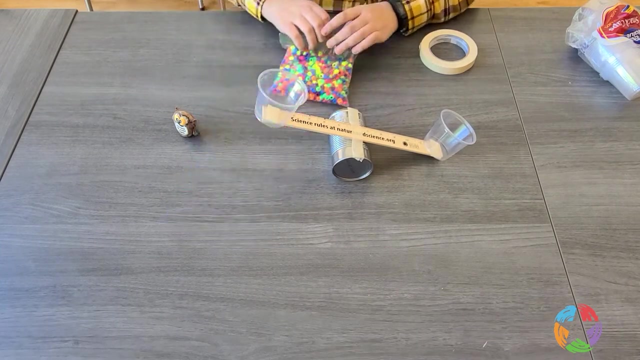 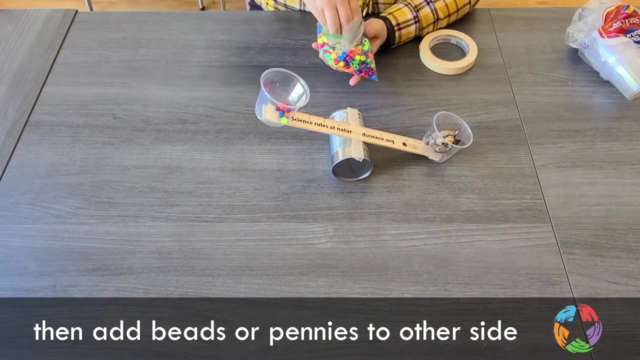 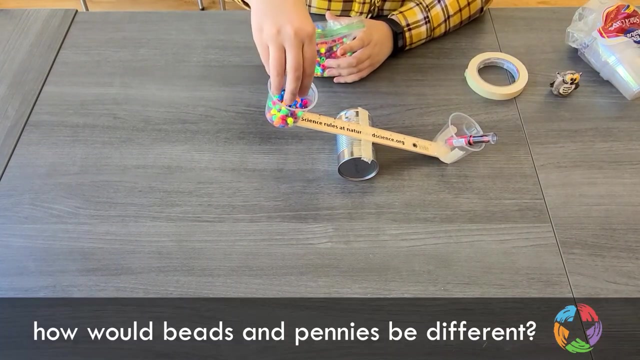 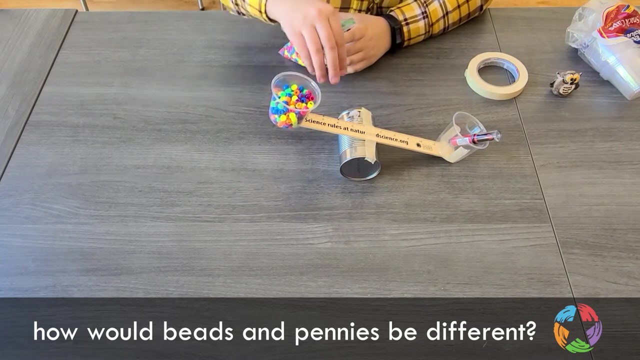 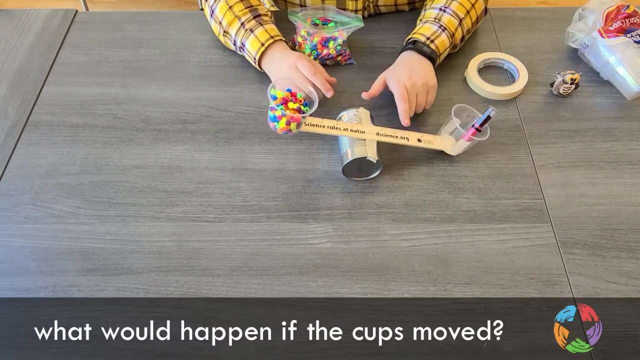 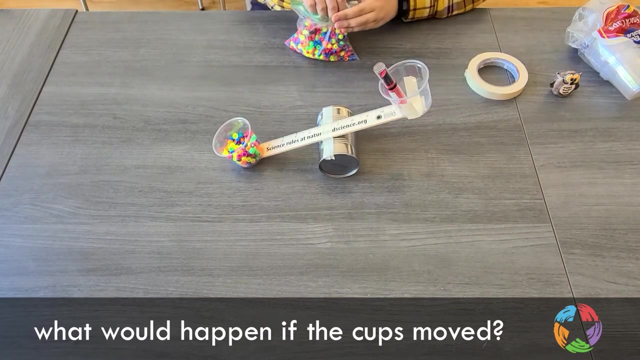 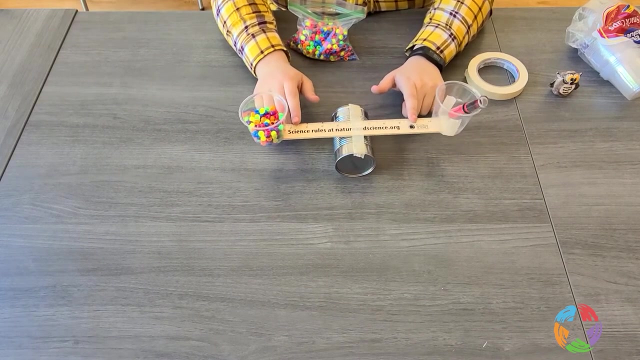 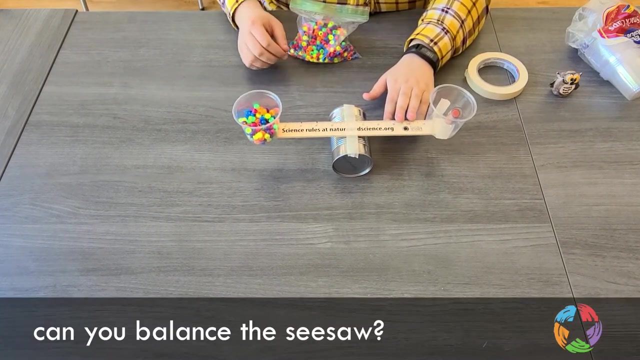 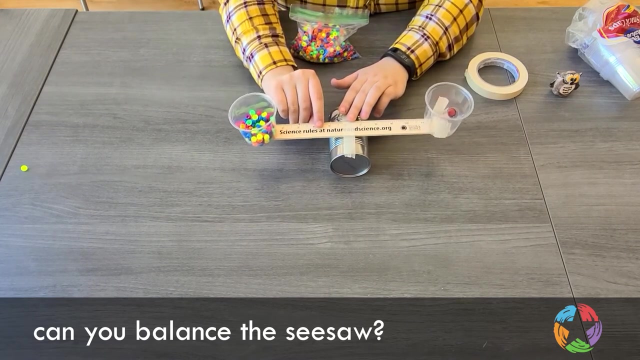 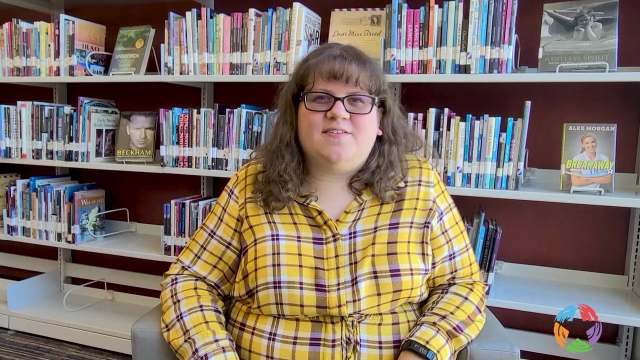 and wheelbarrows. Today we're going to create a small seesaw lever for our toys and see how much effort is required to lift them. So so, so, so, so, so, so. How many items did it take to lift the load? What if we moved the cup from the end to the middle? 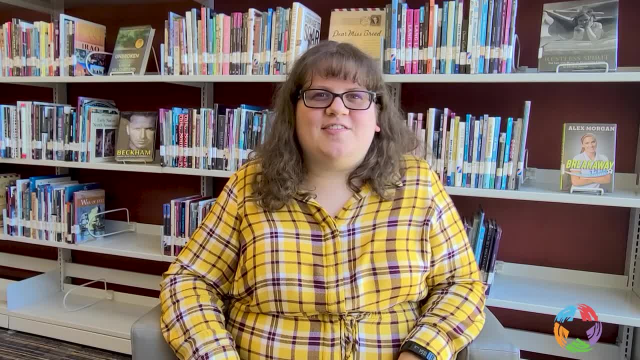 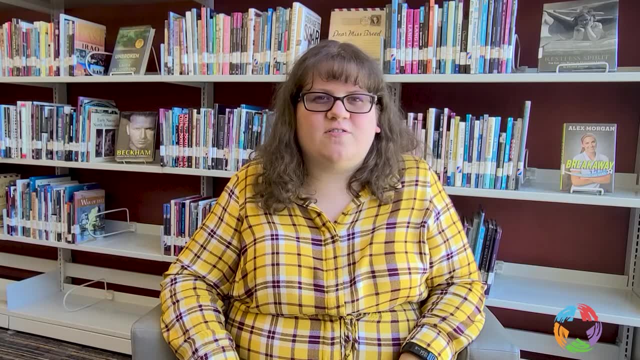 How many would it take? then You can also explore how hard it is to move the seesaw with your finger. Is it easier or harder to lift the load? to lift the load when your finger is on the end of the platform or closer to the fulcrum. 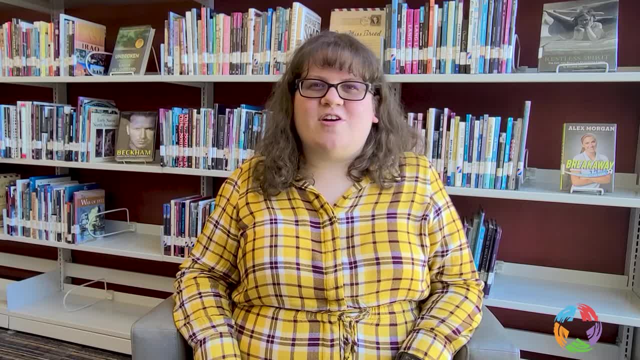 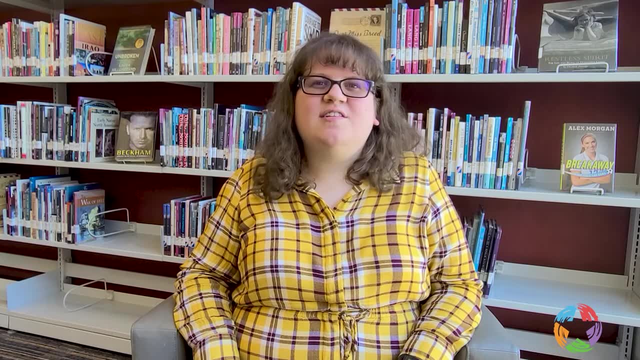 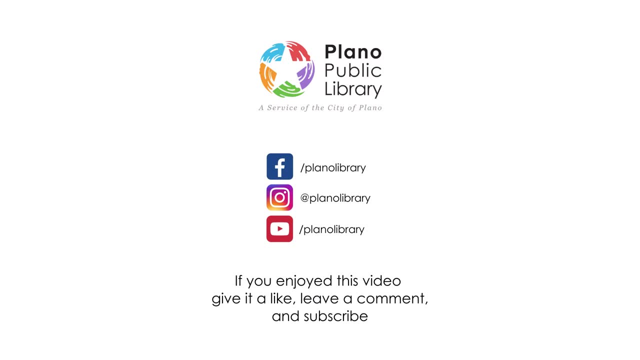 This process of building a simple machine helps unlock the child's imagination. It helps children uncover interests and talents and teaches valuable problem-solving skills and resilience to keep working on a problem until it is solved.